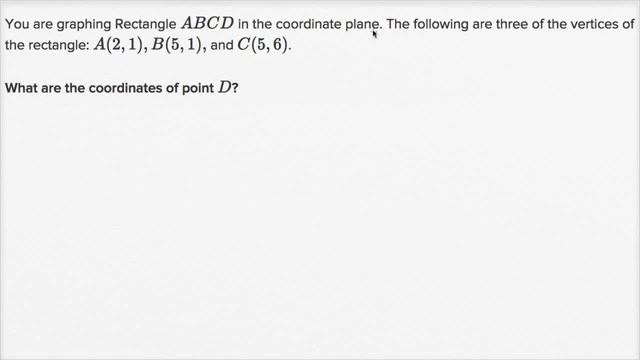 You are graphing rectangle ABCD in the coordinate plane. The following are three of the vertices of the rectangle, And they give us the coordinates. What are the coordinates of point D? All right, well, a good place to start. let's just plot the three vertices that they give us. 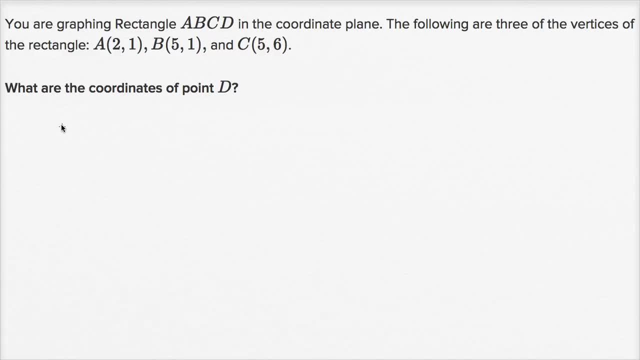 So it looks like they're all in the first quadrant. so I'm gonna focus my coordinate axes on the first quadrant. So that's going to be my y-axis, And let me now that's gonna be my x-axis, And let's see the highest x value that I have. 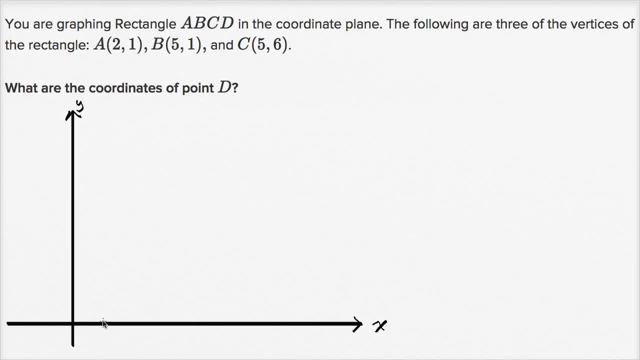 you have a two, I have a five, I have a five. it looks like it goes up to five. So I could say one, two, three, four and five. so that's five. I can just one, two, three, four and five. 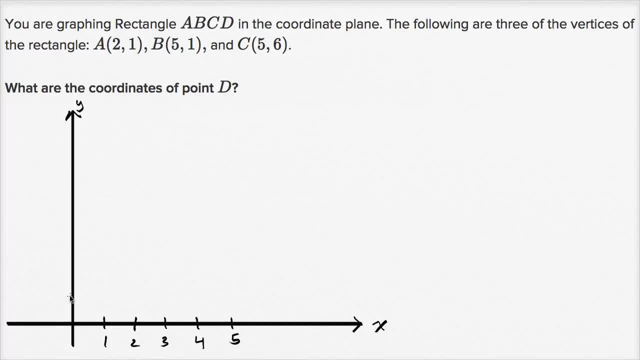 And let's see the highest y value. I have one, one and a six, so it goes up to six. So one, two, three, four, five and six. I can number them: one, two, three, four, five and six. 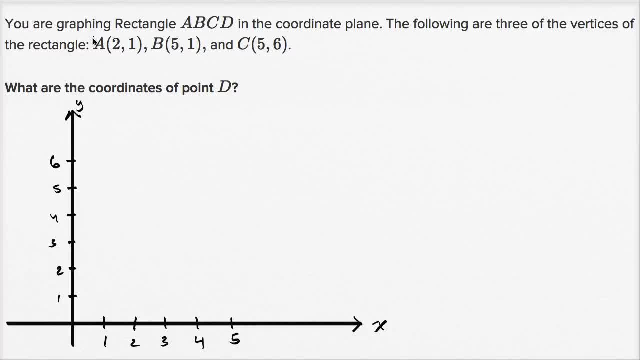 Now let's plot the points. So let's first plot point A, which is at two comma one. X equals two, y is equal to one. So that's that point right over there. Now let's plot point B. Point B is at five comma one. 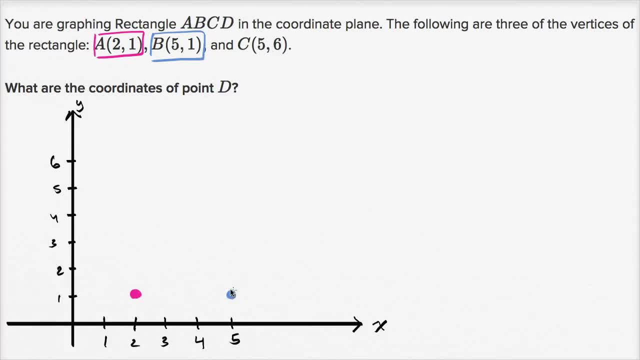 So x equals five, y is equal to one. Okay, That's right over there. Now let's plot point C, Point C- I need to find another color here. Point C is that X is equal to five, Y is equal to six. 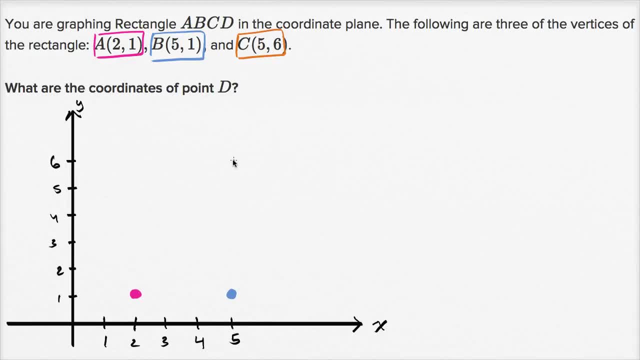 X is equal to five, Y is equal to six, So it sticks us roughly right over there, And so we need to figure out what D is going to be. Well, D is going. this is a rectangle, The sides are parallel, all the vertices. 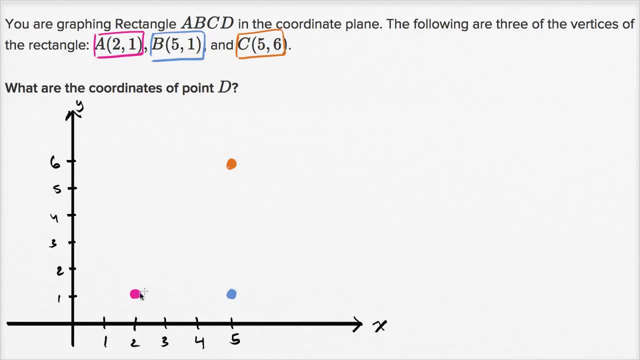 we have right angles at all the vertices. So point D is going to have the same X coordinate as this point right over here. So it's gonna have the same X coordinate. So it's going to have an X coordinate. So let me write this: 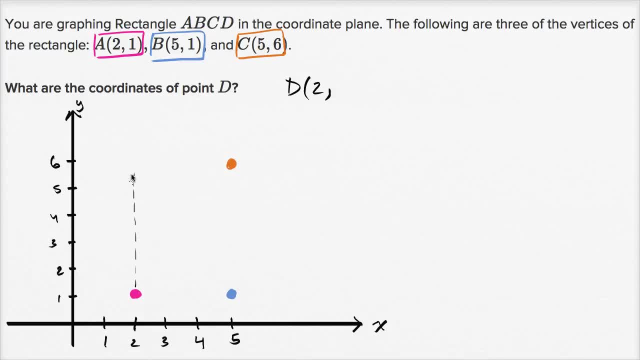 D is going to have an X coordinate of two And it's gonna have the same Y coordinate as this point up here. So it's gonna have a Y coordinate of six of six. So D is going to be at the point two comma six. 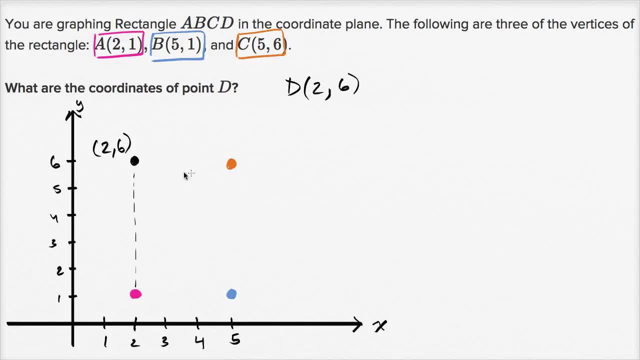 And you see, when we do that, we have set up a nice rectangle here and we can draw the rectangle, So that's one side, that's the top side, that's another side, another side, and then we have that just like that. 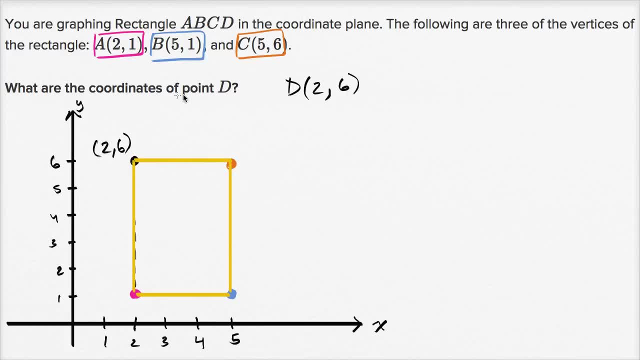 There you go. we have our rectangle, But, most importantly, we answered our question. what are the coordinates of point D? All right, 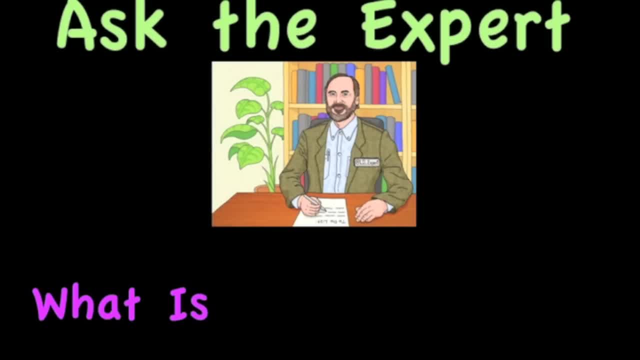 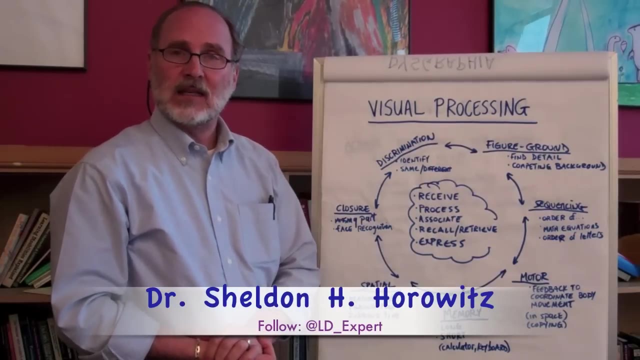 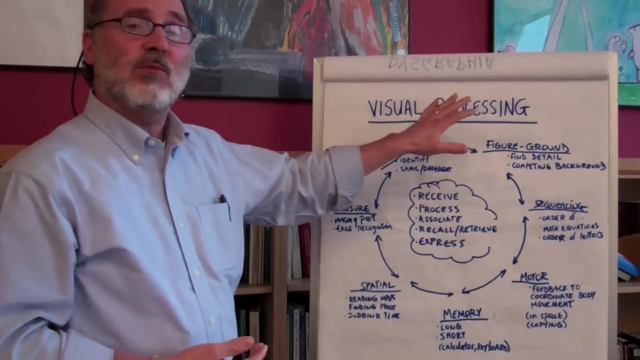 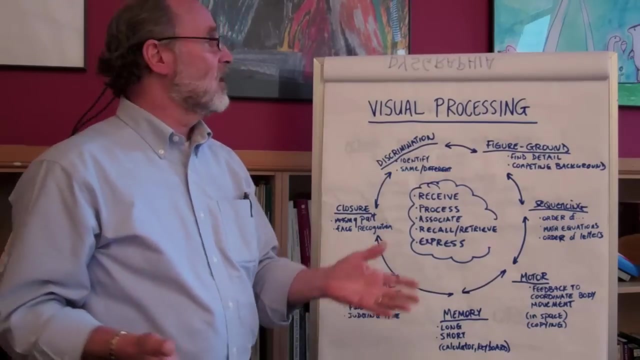 Hi, I'm Dr Sheldon Horowitz here at the National Center for Learning Disabilities. Welcome to the next in our Ask the Expert series. Today, I would like to talk about visual processing. Visual processing is, in and of itself, not a subtype of learning disabilities. 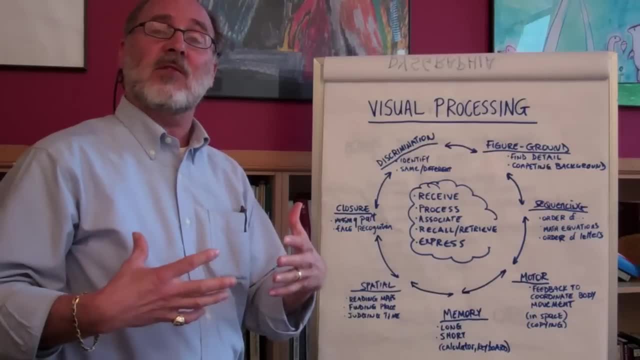 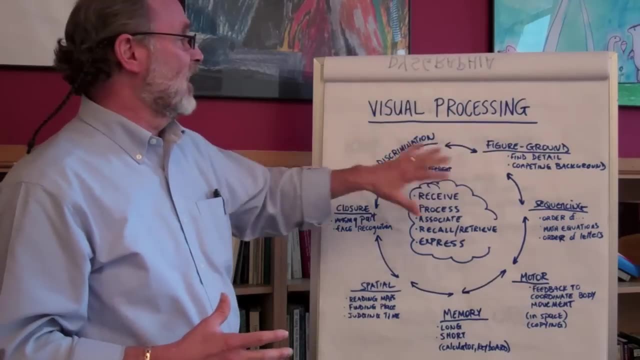 but something that we all do. It's the way that we take information in from our environment and is very problematic for many students with learning disabilities. Let me just provide a little bit of an overview of what we mean by visual processing, First and foremost. 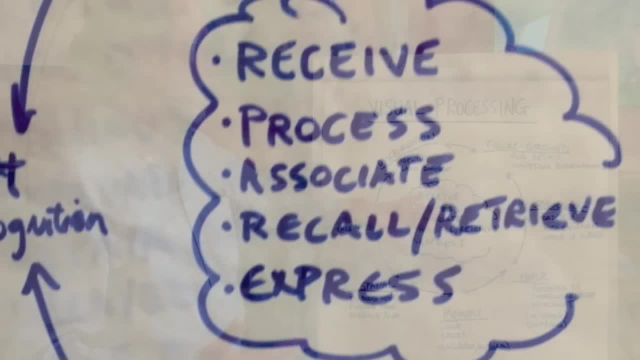 we receive information through our eyes, through our visual sense. That information is then processed, We think about it and we organize it and we understand it in some way. To be able to do something with it and remember it, we have to associate it with some information that